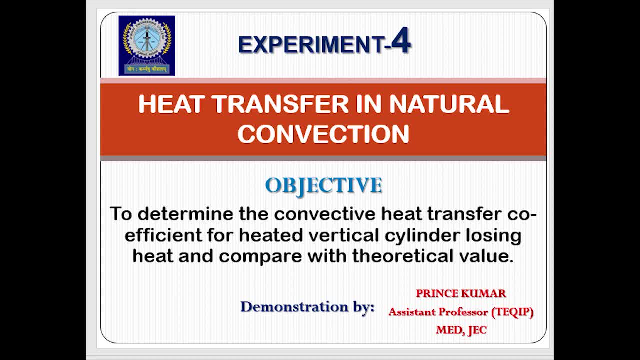 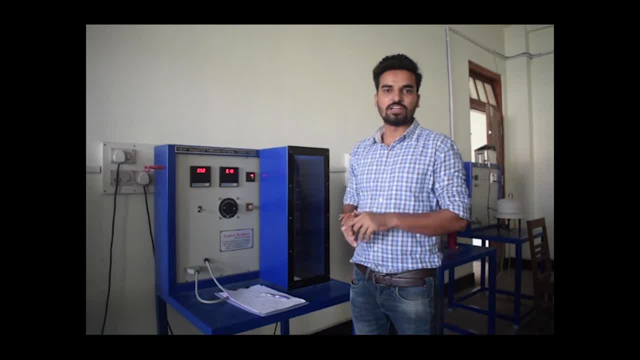 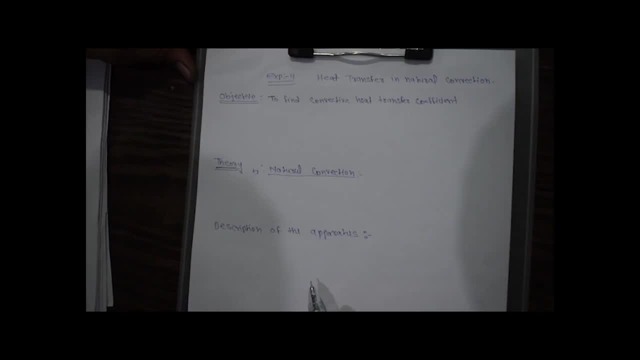 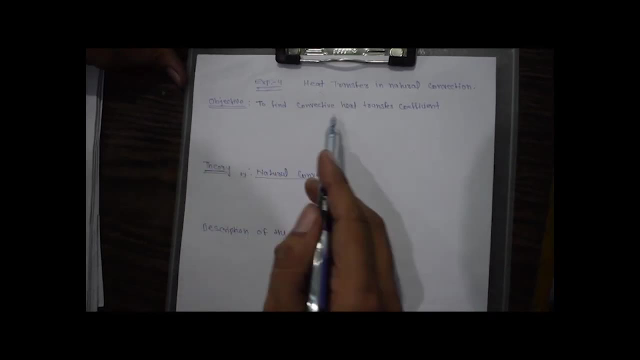 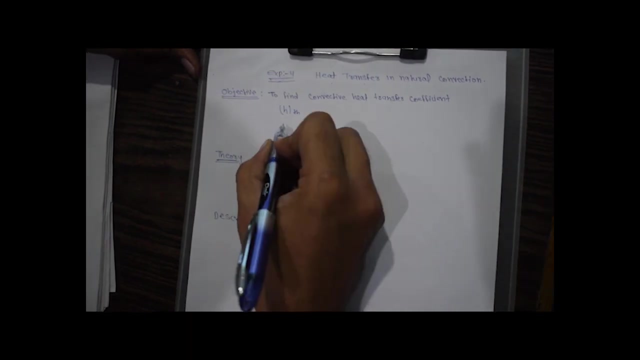 So this is the experiment number 4, heat transfer in natural convection. So our objective is to find out the convective heat transfer coefficient. So our objective is to find out the convective heat transfer coefficient, theoretical and experimental convective heat transfer coefficient. 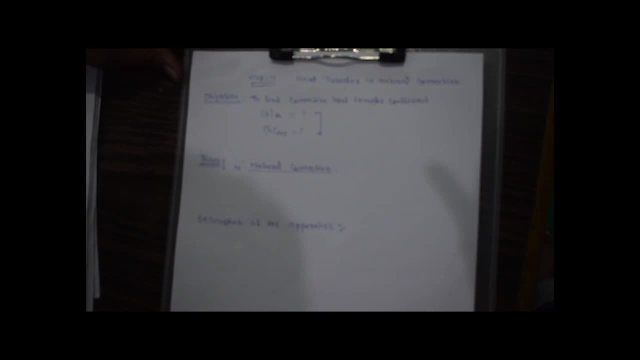 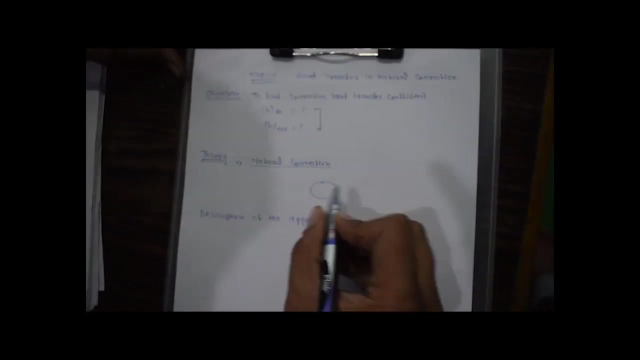 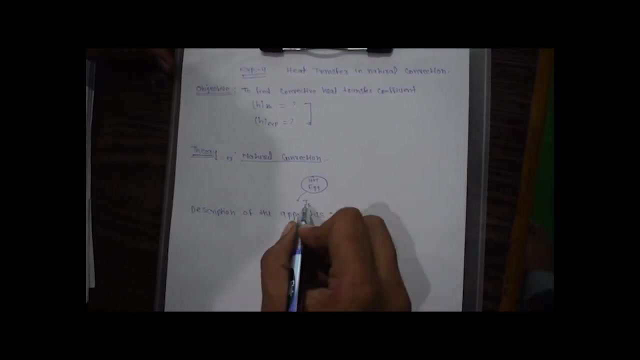 and then we will compare the both. So this is the apparatus of natural convection. So what is the natural convection? Suppose this is the hot air, So this have a temperature T s and this is the ambient temperature. So T s greater than T a, So this surface is at higher. 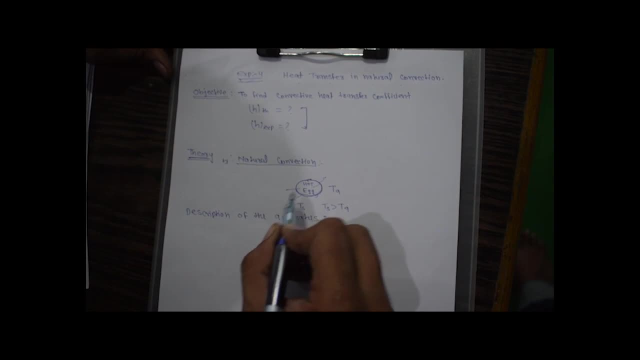 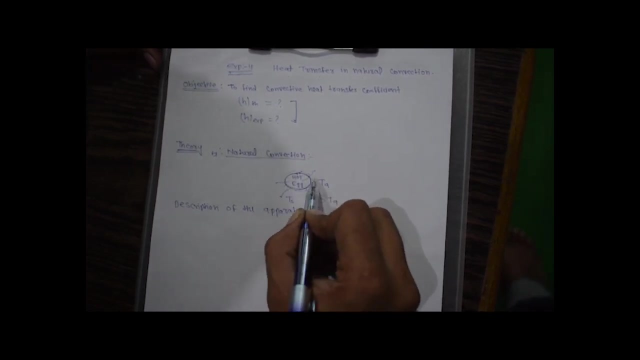 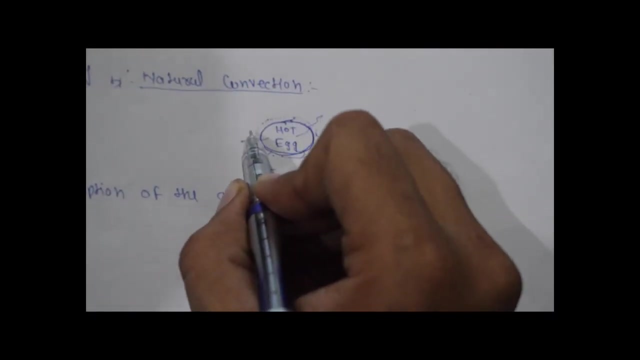 temperature. So heat will transfer to the environment and the nearby air get heated and due to this the temperature of nearby air will increase So that the density of the air will decrease. So if the density will decrease, then that air will lift upward, That air will. 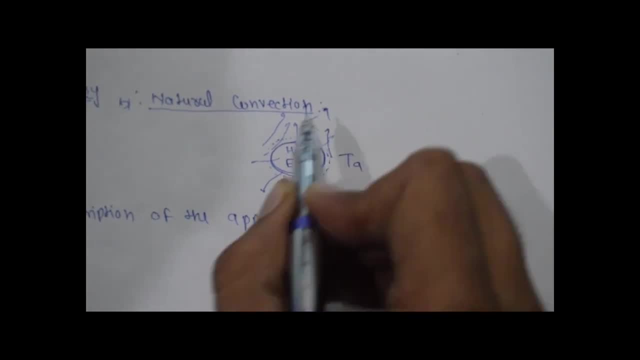 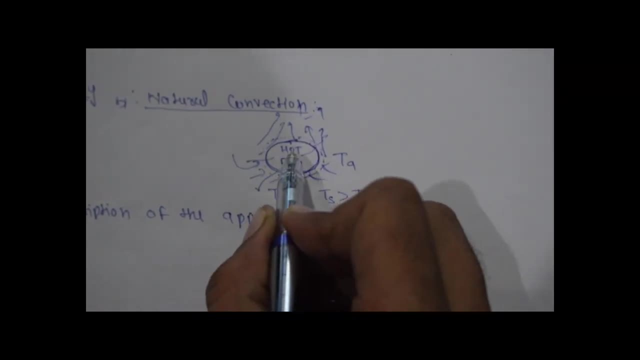 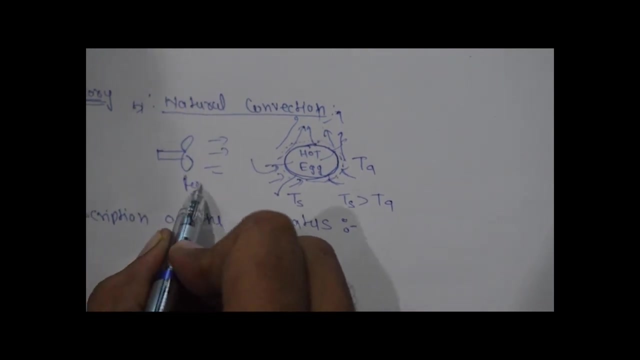 require a temperature of constant temperature. So if the density of the air will be increased, then we do not have heat transfer of the weather heading on the round, So we do not have liquid warm air, So the temperature will also increaseopers effeq speeches. So the temperature of the water? 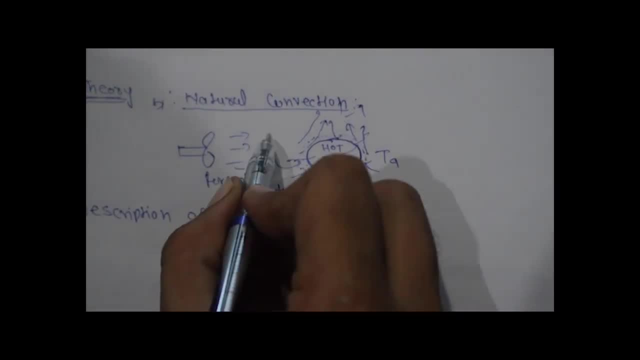 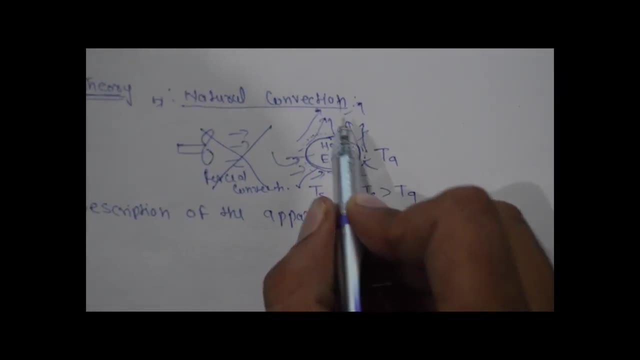 that we pour can be increased. So local LocOGC for case, we are not using any external agency. so this is the natural convection. now this is due to by the effect of buoyancy force. so what is the description i am showing here in the apparatus? 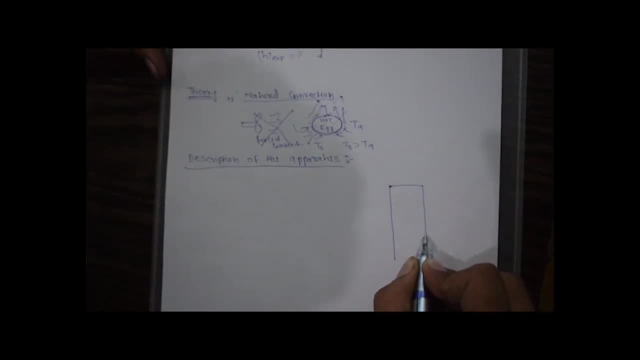 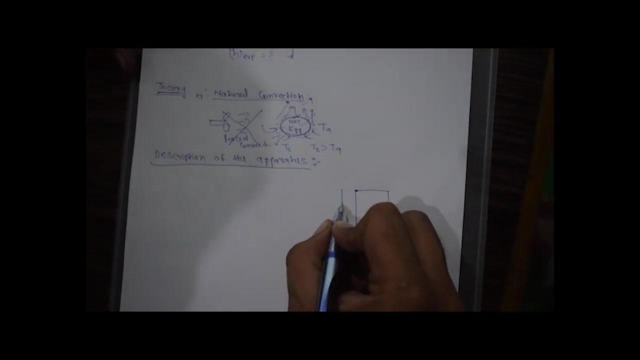 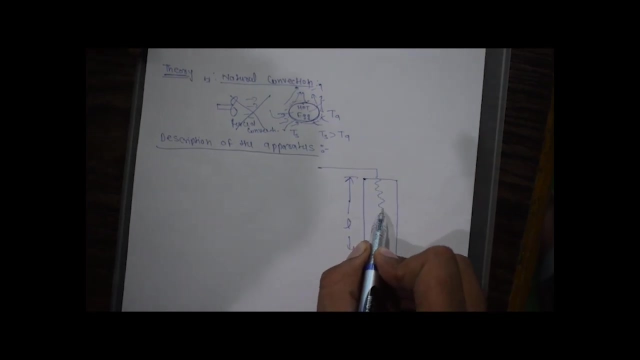 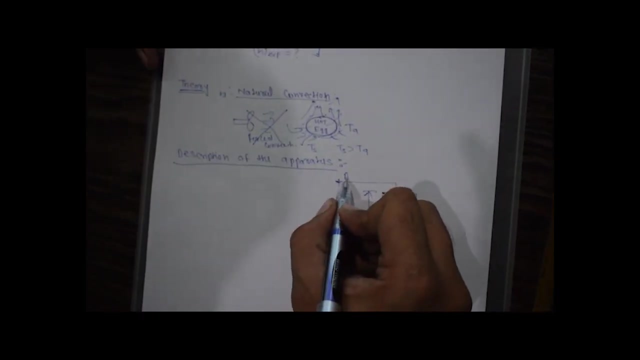 so there is a one cylindrical pipe. there is a one cylindrical pipe diameter d. diameter d and length is l. length is l. so inside this slender a one heater is clubbed and that heater- this will con that heater- is connected to the alternating current. when we switch on the current, the 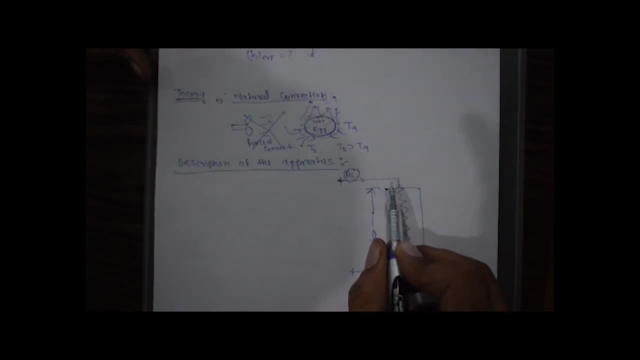 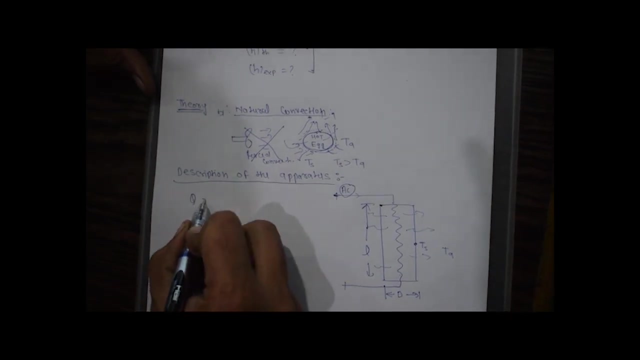 current will passing through this heater and the, and the electric energy will convert it into the heat energy and that will dissipate to the environment from the surface of the slender. so suppose at a time the surface temperature is ts and the ambient temperature is ta, so the heat transfer according to newton's law of cooling, according to newton's law of 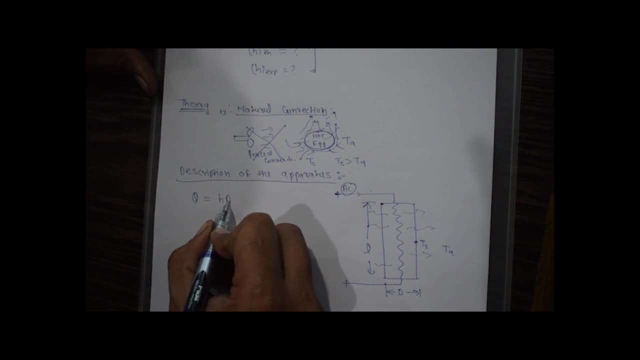 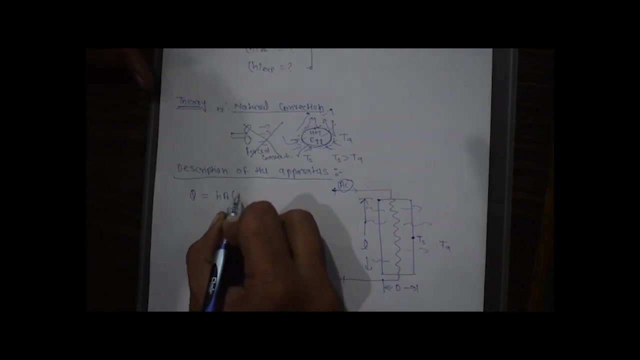 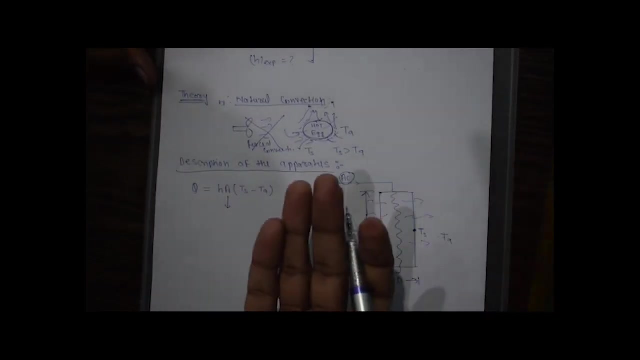 cooling, that is equals to h convective heat transfer coefficient, area of the slender and the temperature difference. so this is the temperature difference, so this is ts minus ta. so this is the area area, the cylinder. so we have to take the surface area because the heat is transferred. 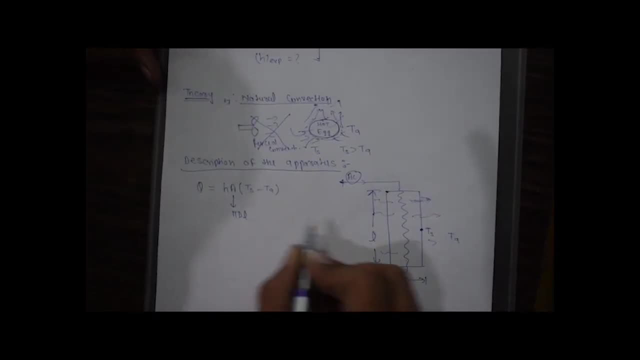 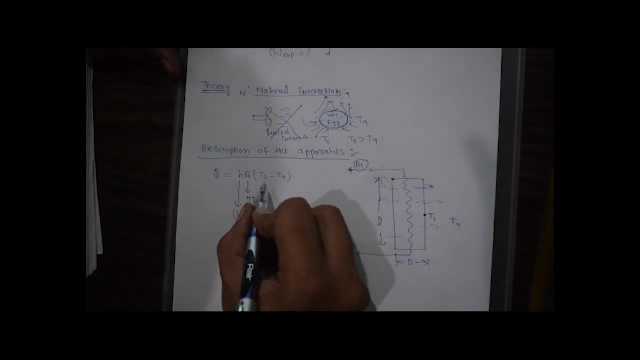 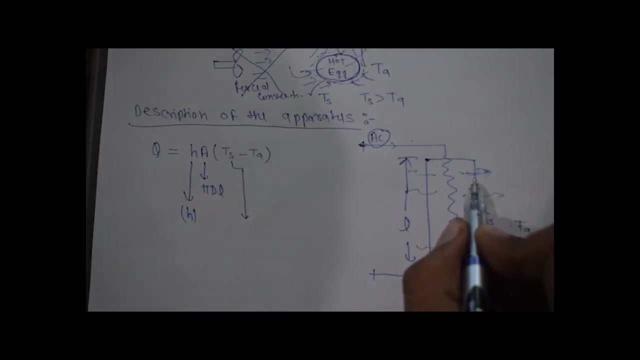 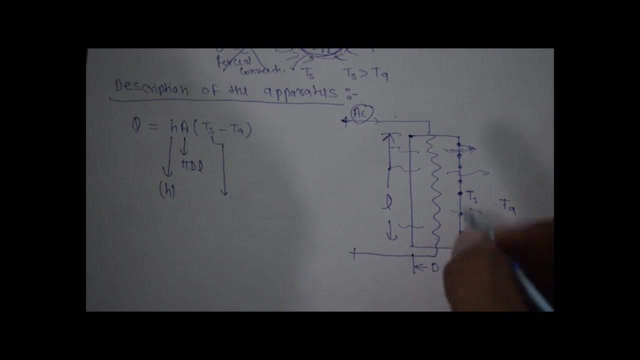 from the surface. so this is pi d and the length of the cylinder. this is the convective heat transfer coefficient h. this is the surface temperature. this is the surface temperature. to measure the surface temperature, we installed the seven thermocouple. we installed the seven thermocouple on the surface. to measure the surface temperature, we installed the seven. 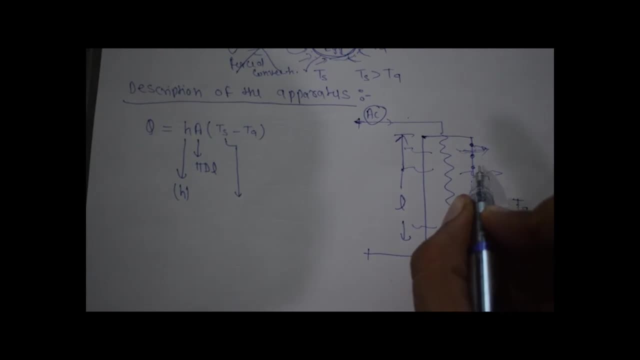 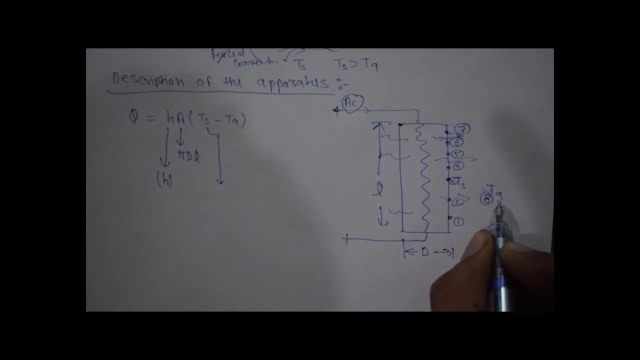 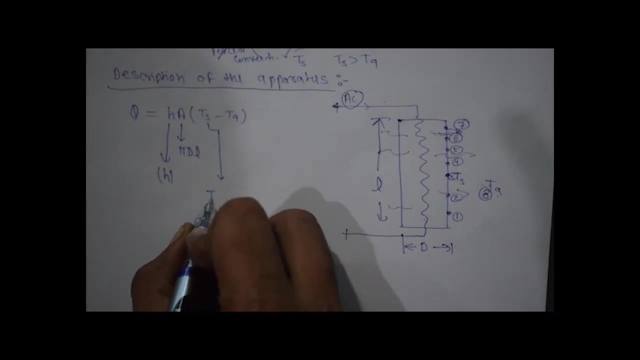 thermocouple 1, 2, 3, 4, 5, 6 and 7 and 1 thermocouple, number 8 is used to measure the ambient temperature. so the surface temperature is given by the average of these 7 thermocouple. so ts equals to: 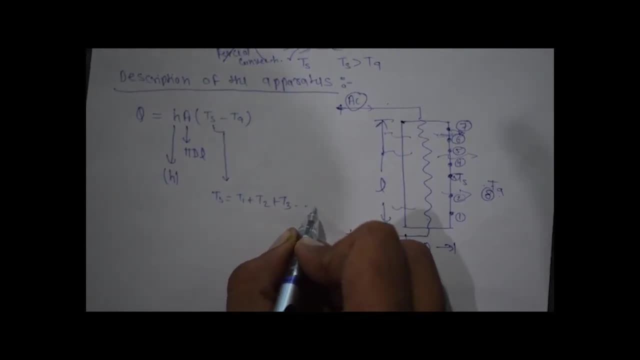 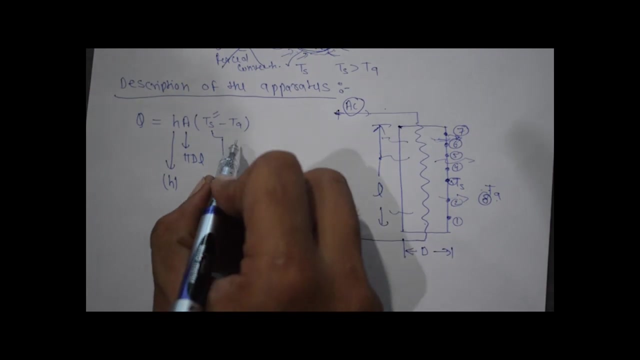 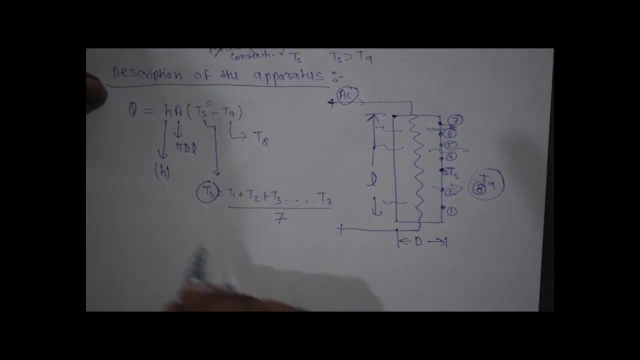 t1 plus t2 plus t3 up to t7. if we find out the average, we get the surface temperature and the ta is given by the 8 thermocouple. so this is the reading of 8 thermocouple number 8 and the heat input. heat input is equals to the voltage and the current. 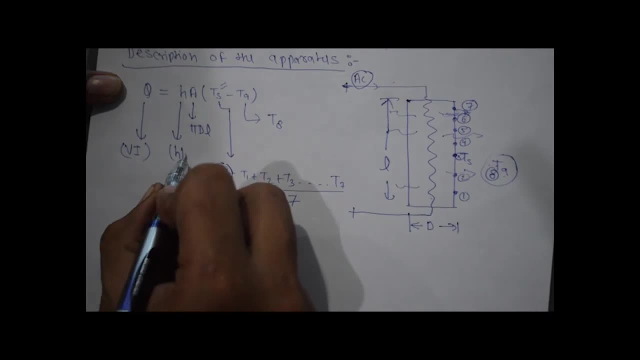 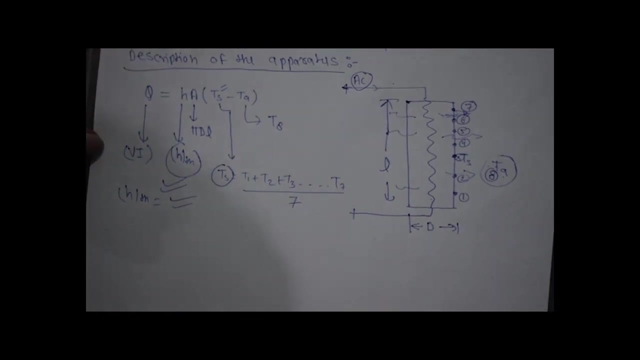 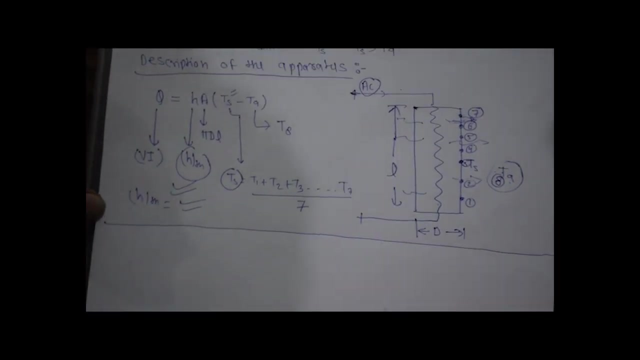 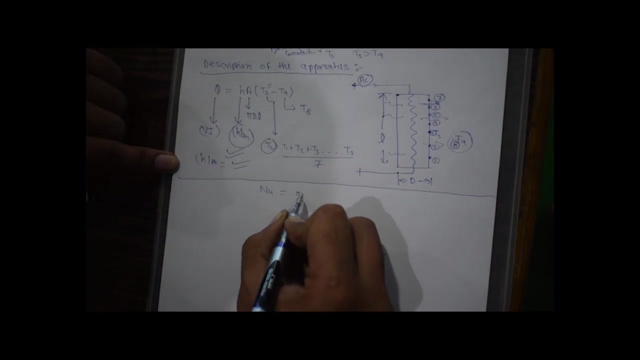 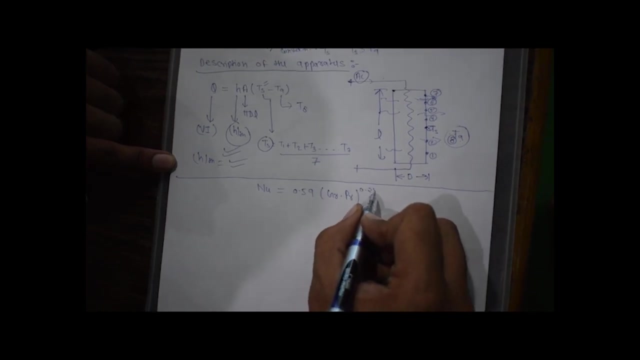 so from here we get the, we get the theoretical convective heat transfer coefficient, but we also we have to also find out the experimental heat transfer coefficient. so for that, for the natural convection, there is a one relation, non-dimensional relation, that is nu: 0.59 gr, dot pr, power 2.5. so this is the nusselt number and that is given by 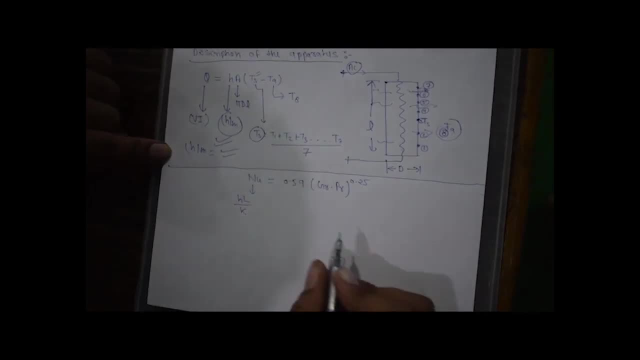 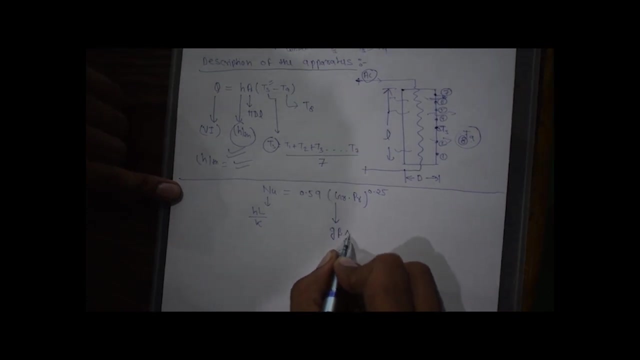 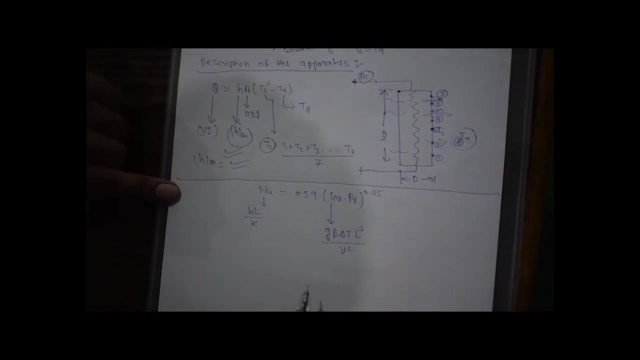 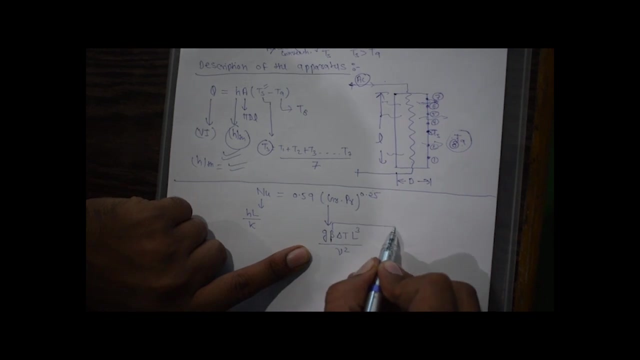 h, l by k, this is the 0.59 and this is the grasshopper number and that is given by g, beta by k, delta, t, l, cube by nu square. so this is the exhalation due to gravity and this is the beta and 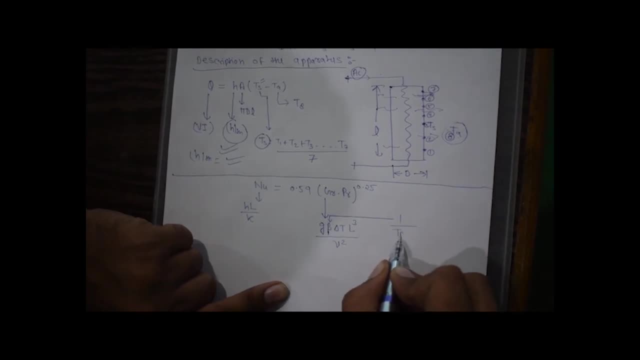 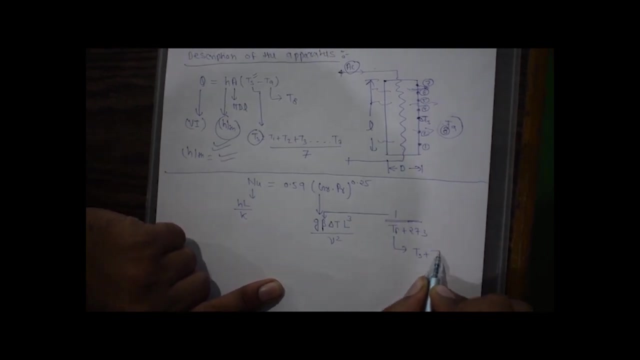 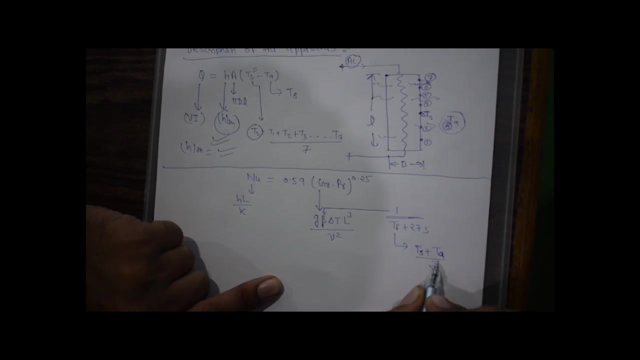 this is equals to. this is equals to one by tf plus 273. so what is the tf? tf is nothing, but this is the average temperature of ts and ambient. This is in. this will come in degree Celsius, So we have to add 273 to convert it. 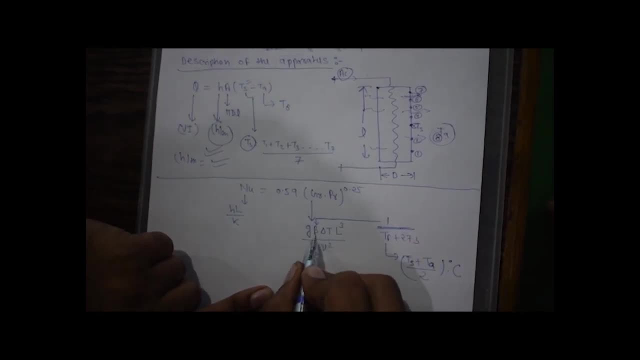 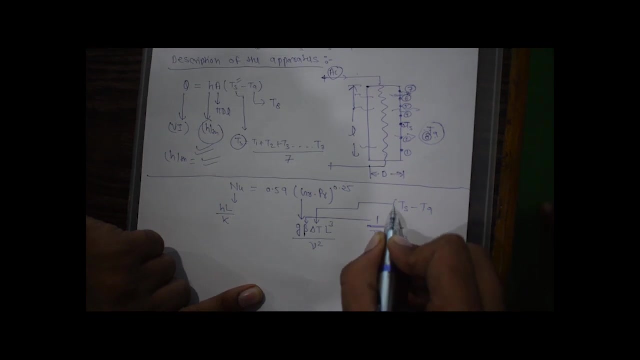 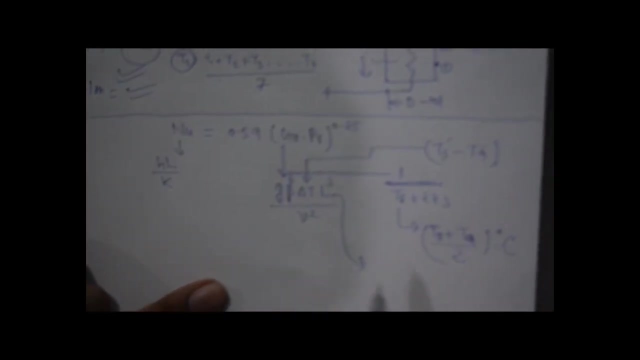 into the Kelvin and by reciprocal of this we get the beta value of beta And delta T is again. delta T is nothing, but this is the T s minus T a, T s minus T a we get from the readings of thermocouple T s and T. a And L is nothing, but this is the. this is the characteristic dimension. 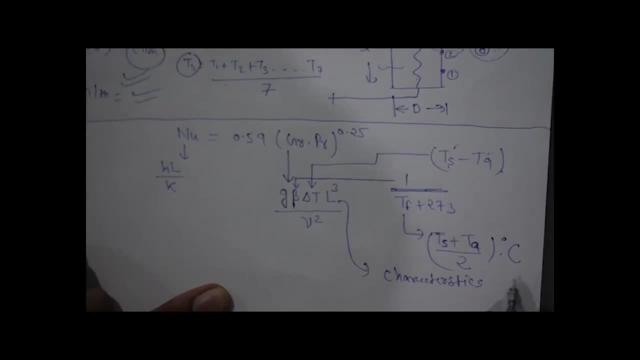 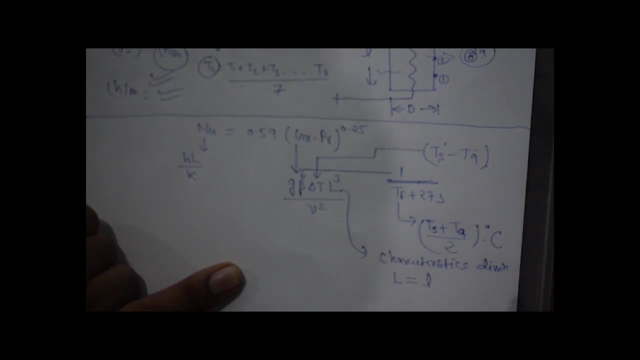 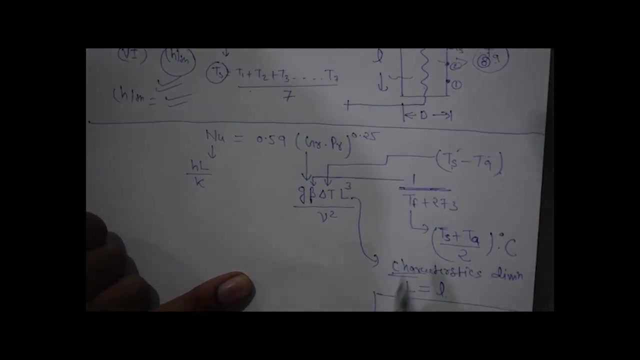 So characteristics, dimensions, and that is given, that is L equals to L. This is for the cylinder. For the cylinder, characteristic dimension is already defined. This is equals to the L. Suppose, instead of the, instead of this cylinder, there is a sphere. So for that condition, 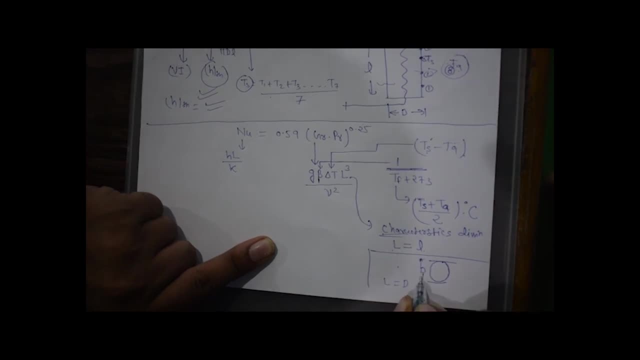 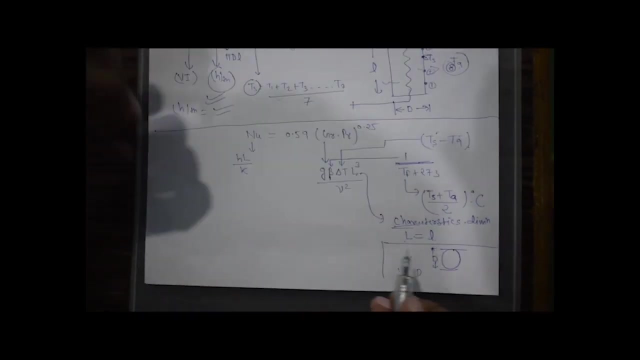 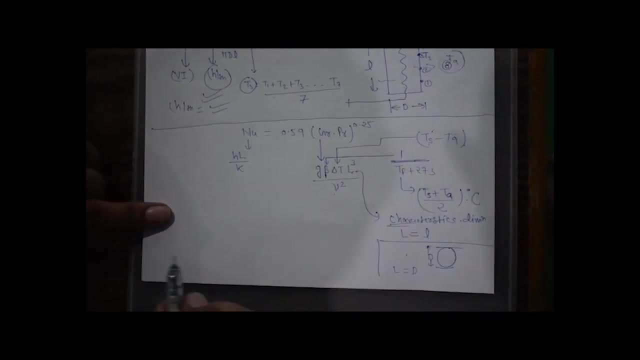 L equals to D. D is the diameter of that sphere. But in this apparatus there is a cylinder, So characteristic dimension equals to the length of the cylinder. And so we got this, this, this one and also L. Now the. this is again the characteristic dimension. So we we have to find 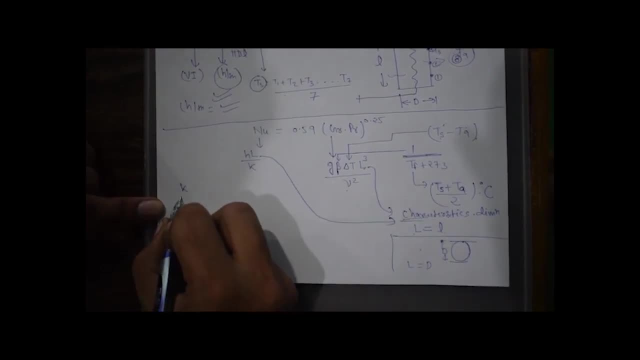 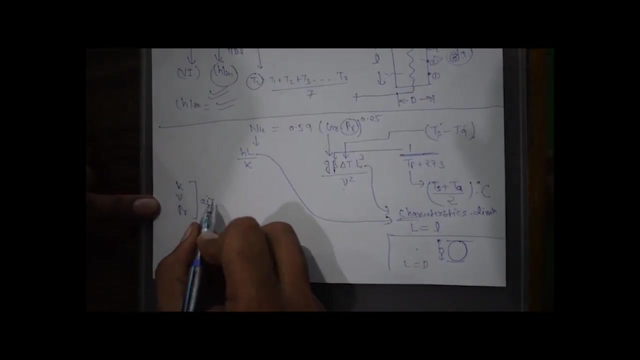 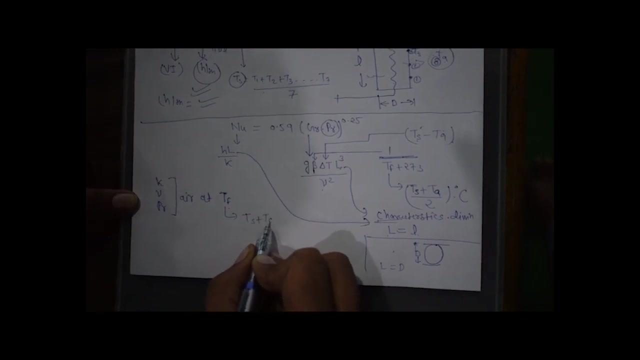 out the K and nu and also Penter number. These all are the property of air at at this temperature, T f. So T f is T s plus T a by 2. So we have, we have to take the property of air from the. 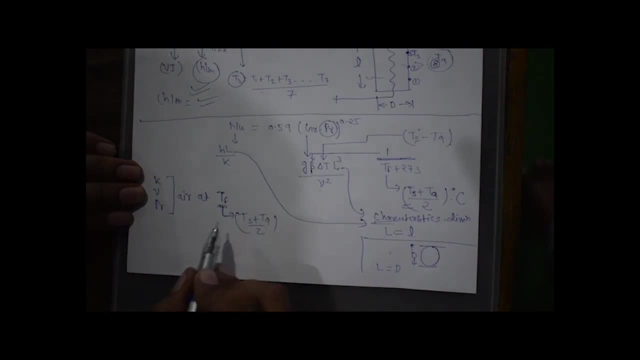 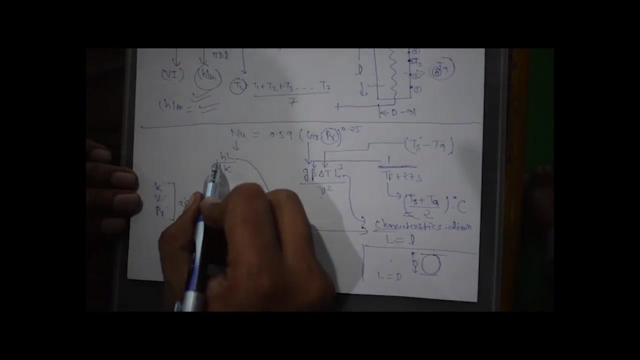 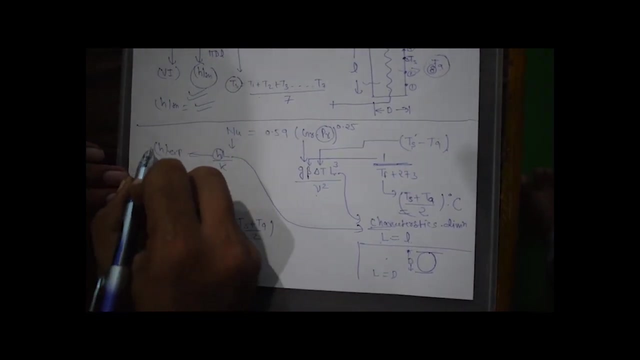 table, air table at T f temperature. So we already, we can easily find out these things. So there is a one unknown only. So this is the convective heat transfer coefficient, experimental convective heat transfer coefficient. So from the apparatus we got the all the. 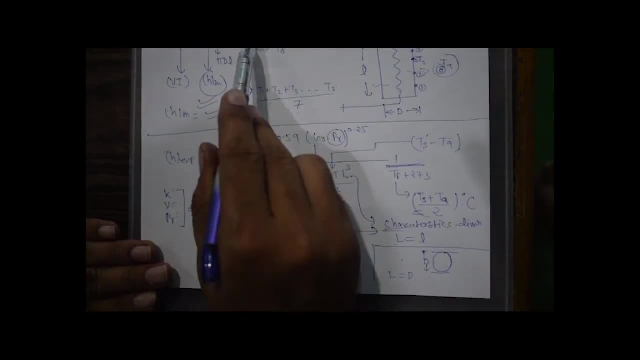 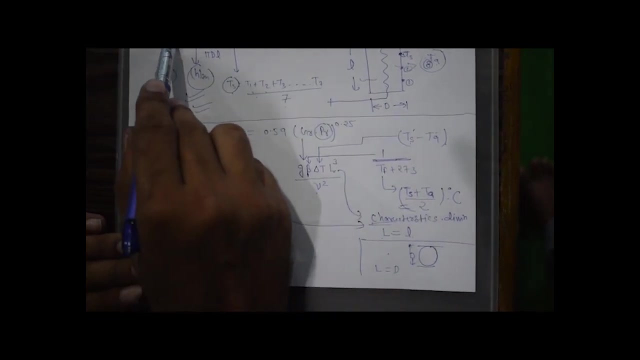 temperatures And we can easily find out the surface temperature and ambient temperature And area is also given, because the length is given and diameter is given And this is the heat input That is equals to V. into I we put this, we get the convective heat transfer coefficient. 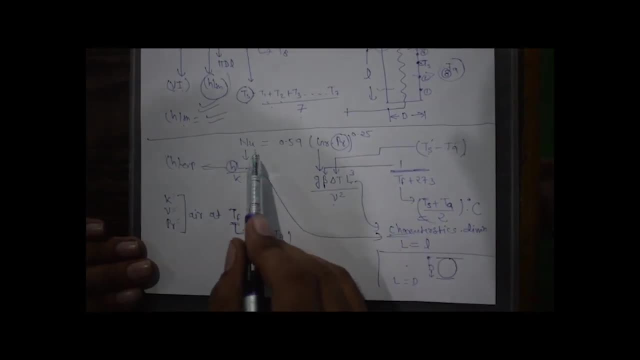 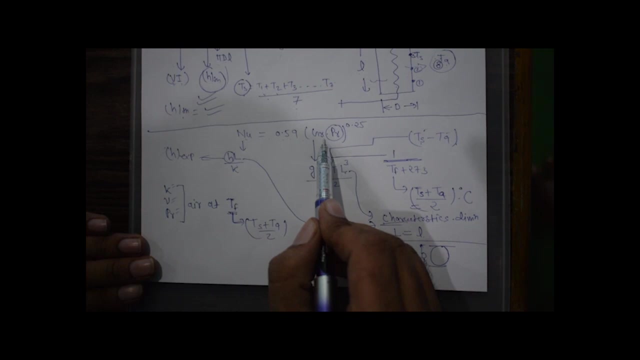 theoretical convective heat transfer coefficient And for the experimental we used, we used this non-dimensional relation. This is the Nusselt number. Nusselt number equals to point five nine Grassoff number and this is the Prentel number And the power. 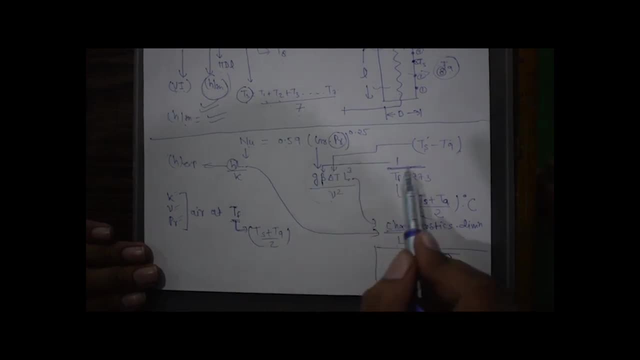 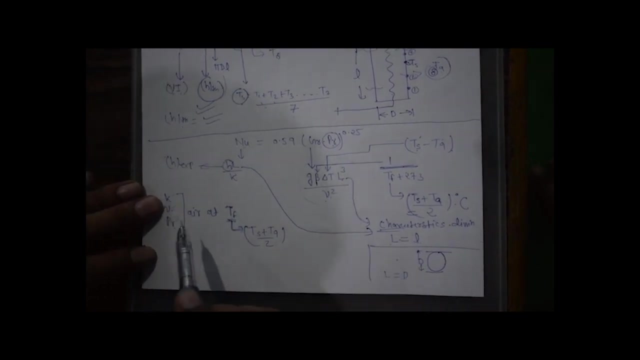 is 0.25.. So from here we get the desktop number and parental number. we get from the air table at temperature T, f and nu and k also we get from the air table and we can easily find out the convective heat transfer coefficient, experimental value. So after: 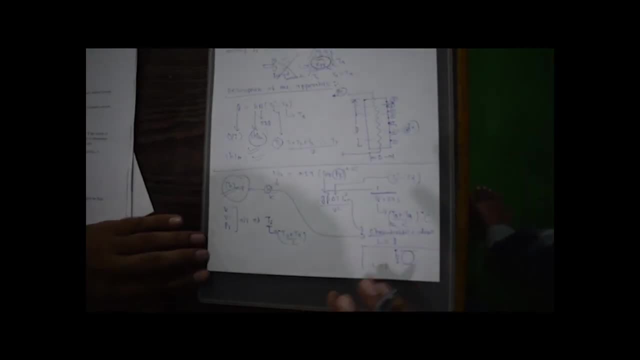 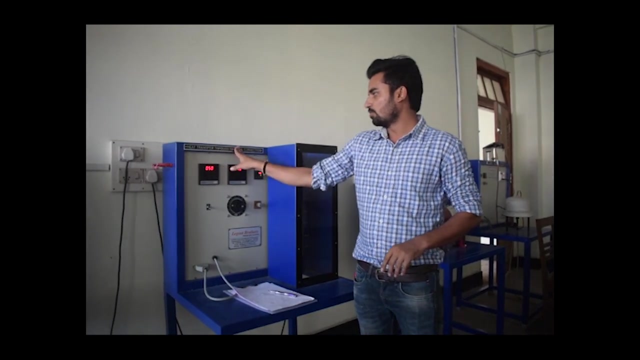 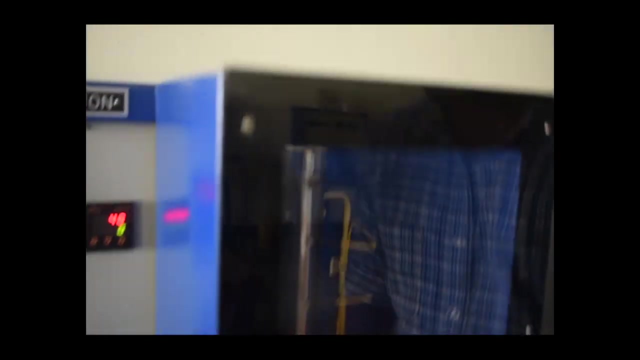 that we can compare both. So let us see how to get these values from the apparatus. This is the apparatus: heat transfer through natural convection. So this is a major one cylindrical pipe, This is one cylindrical pipe and these are the seven thermocouple. 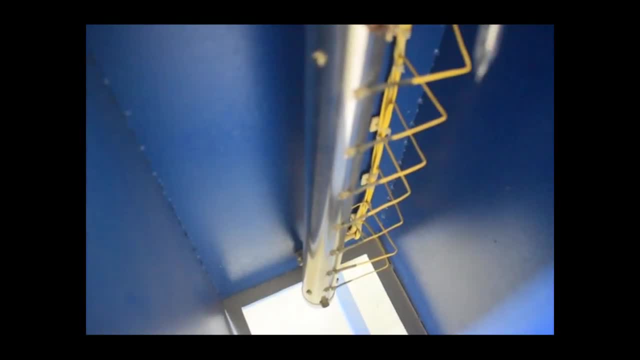 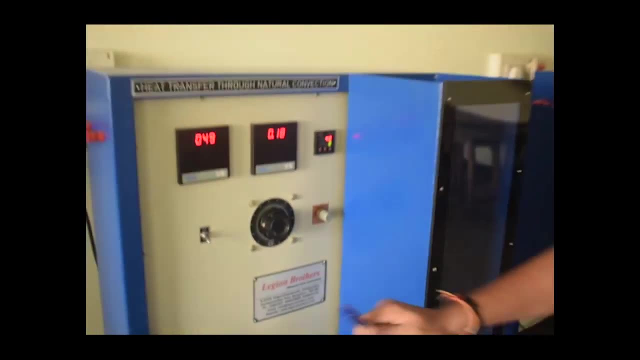 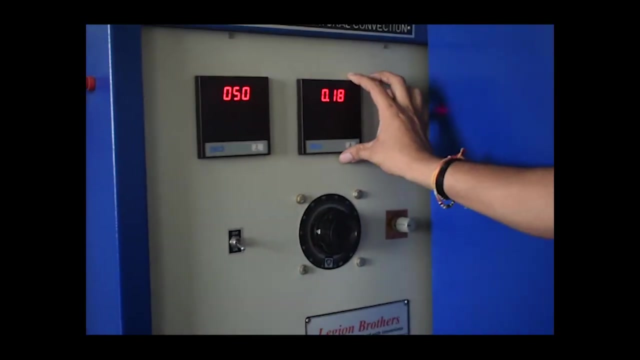 which I already described. These are the seven thermocouple and one thermocouple is open to measure the environmental ambient temperature. Okay, First turn on the main switch. First turn on the main switch and now give the power input. This is the voltage meter. This is the current meter. So by adjusting, 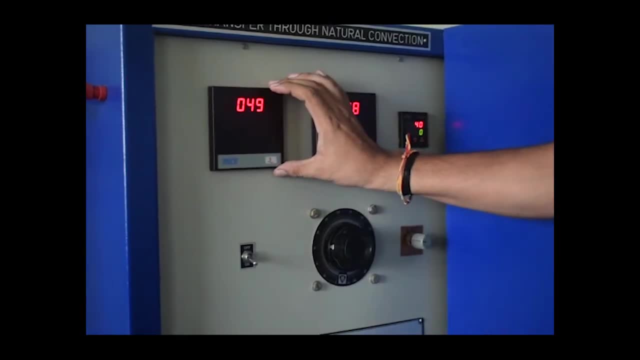 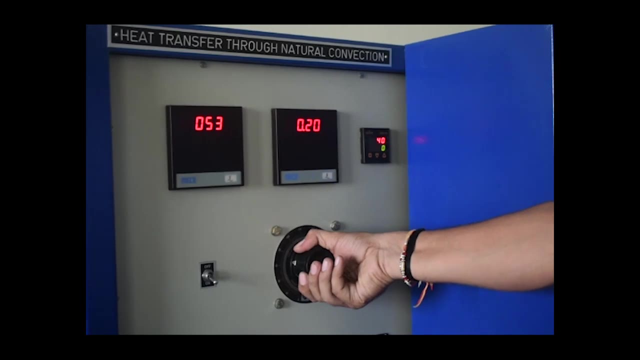 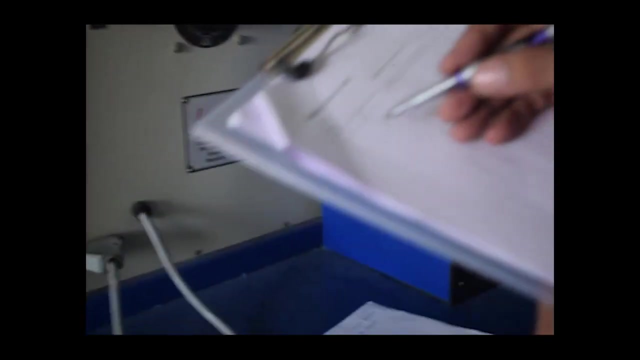 this now. according to that, we get the voltage input. So according to the voltage, there is a current You will show in this meter. So I already said it on 50 volt. Okay, This is our observation. This is our observation table. So after giving the power input, after: 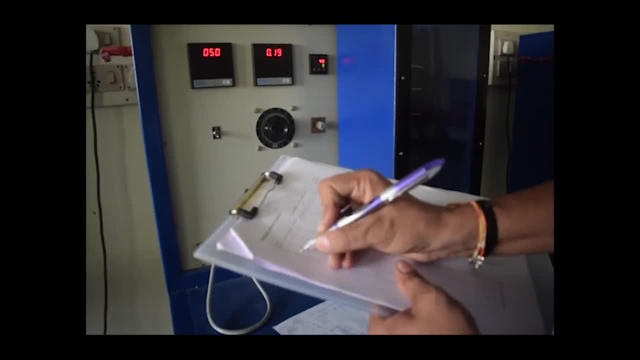 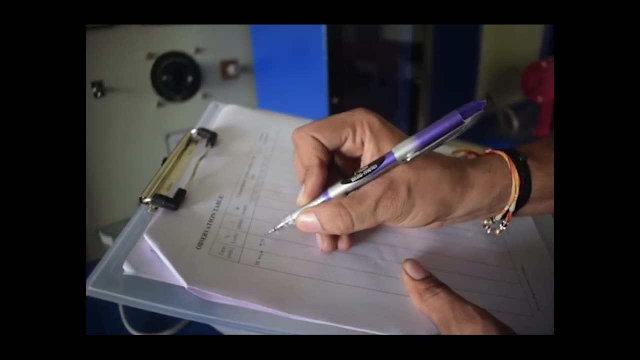 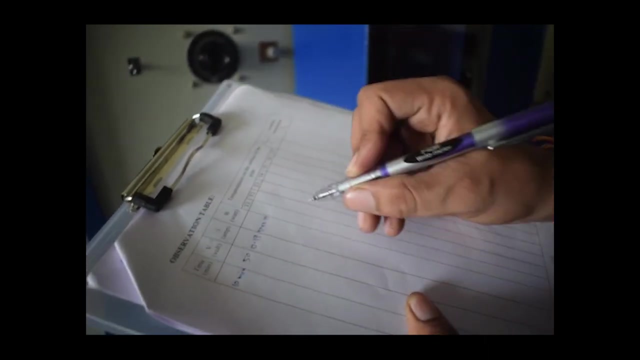 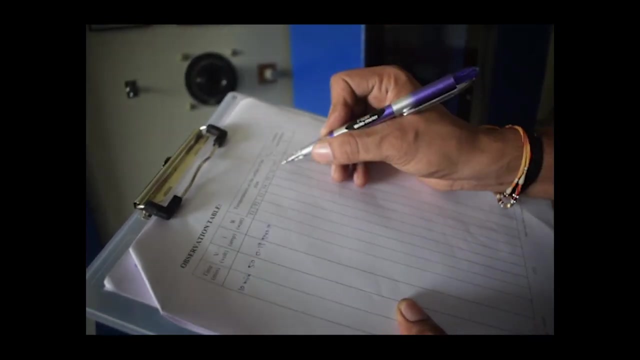 10 minute. we have to take the first reading, First reading, after 10 minute, After 10 minute, the first reading. So voltage is suppose 50.. After 10 minute and current is 1.9. And 50 into 0.19 is the power input. T 1, T 2, T 3, T 4, T 5, T 6 and T 7 are the 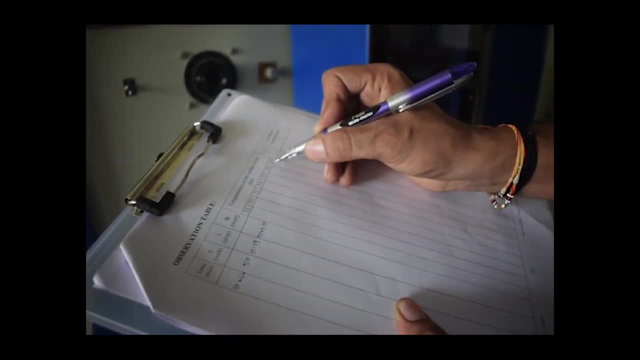 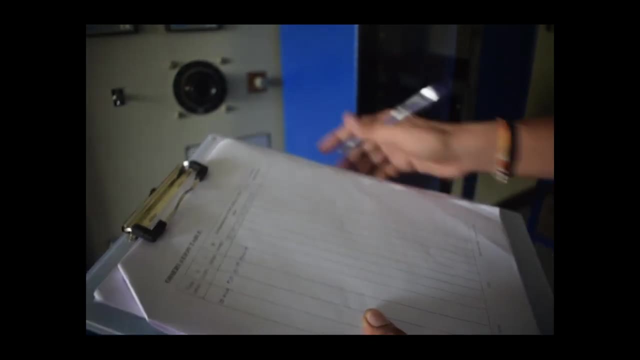 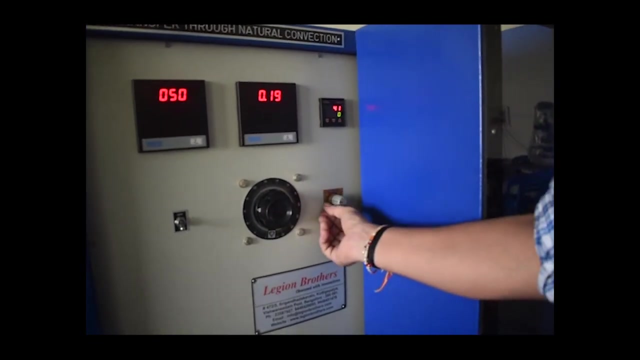 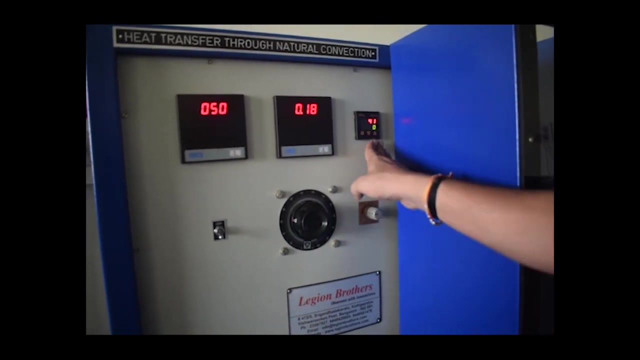 temperature of thermocouples. If we take the average of these 7 thermocouple, we get the surface temperature. So, Okay, out the temperature. so there is a one. now, by adjusting this there is a notation one to eight. so by adjusting this we got the temperature in this display. so this is at t, at t1. this is at t1. 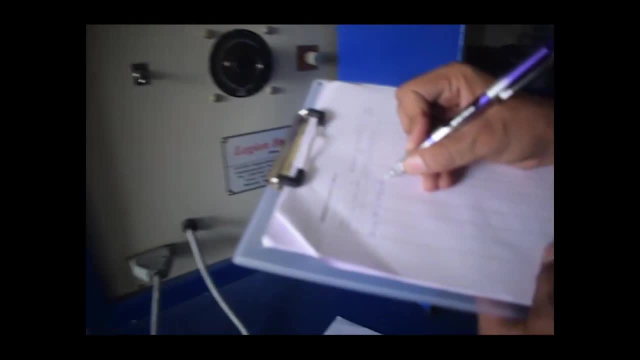 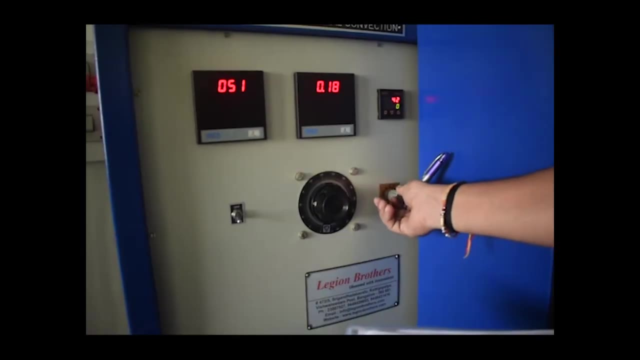 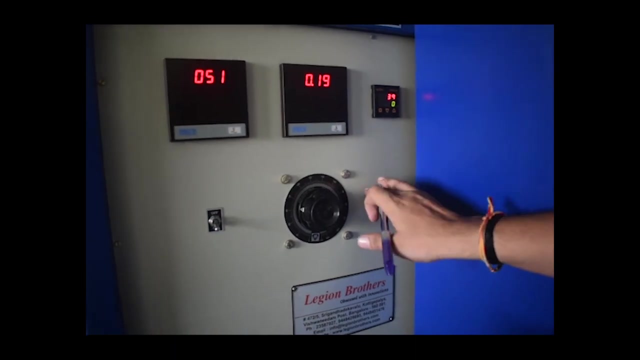 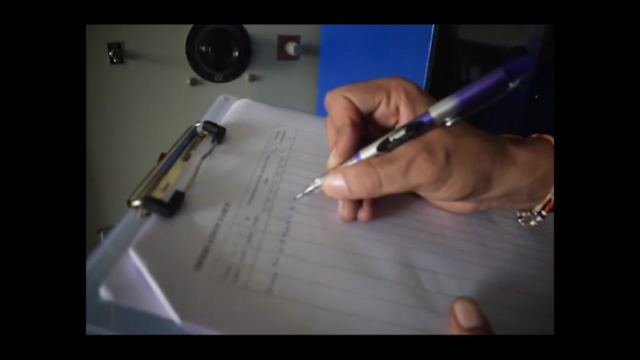 so this is the temperature of first thermogabal. this is 41. if i rotate this, this will give the temperature of t2 and then t3, t4, t5, like that we got the reading of all seven thermogabals. just note down the reading. suppose this is 41, this is 41. this is 40. this is 40, this is 39, this. 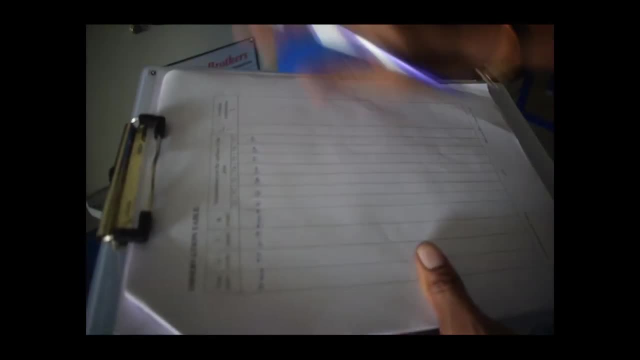 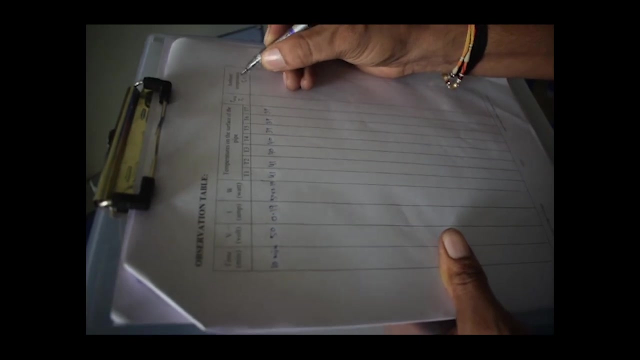 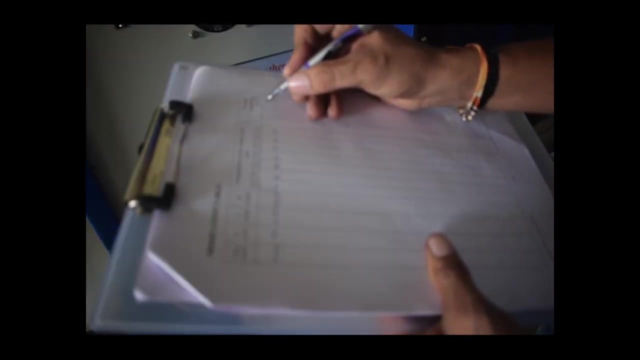 is 39. this is 39. these are the reading we got from the apparatus. suppose these are the reading okay, and the ambient temperature. this is t8, okay, okay. the eighth reading is the reading of thermogabal for the ambient temperature. suppose this is the 30. 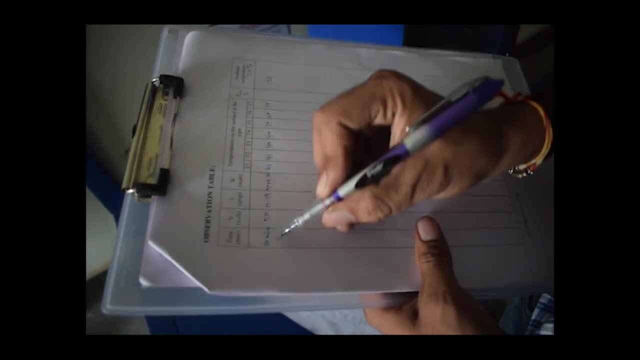 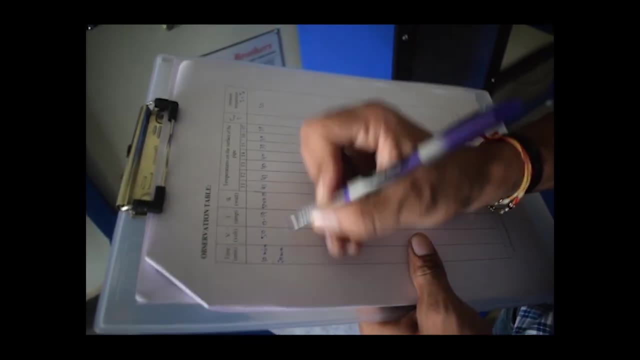 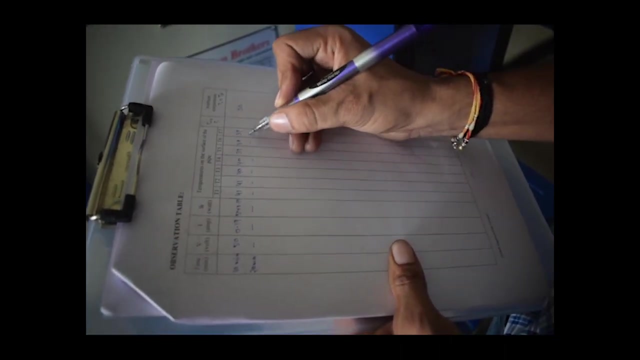 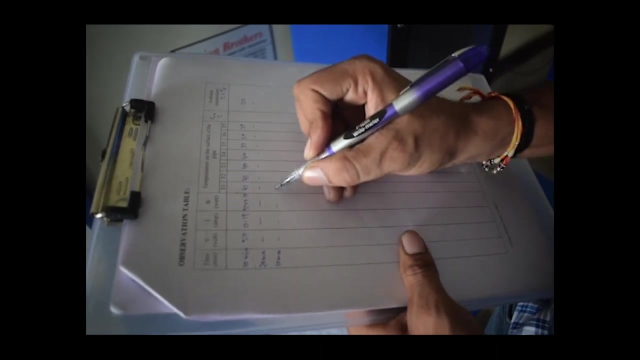 okay, this is our first reading at 10 minute from the beginning. now take the another reading after 10 minute, so from the beginning this is 20 minute. so according to that, note down the voltage current and note down all the temperature by adjusting the temperature. now, then again take the reading after 10 minute. suppose these are the readings. 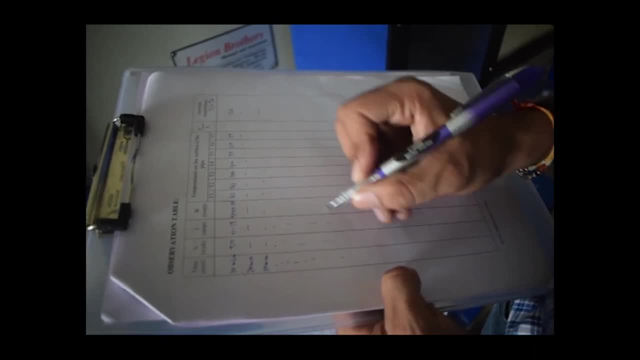 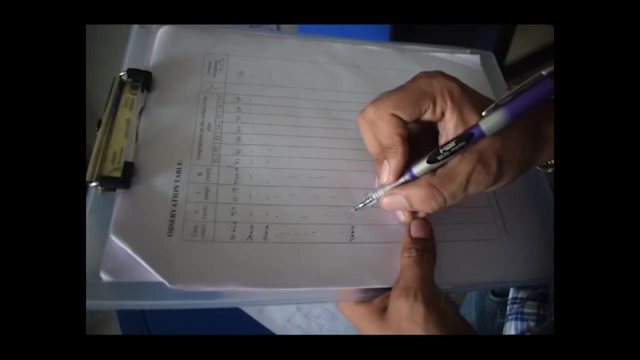 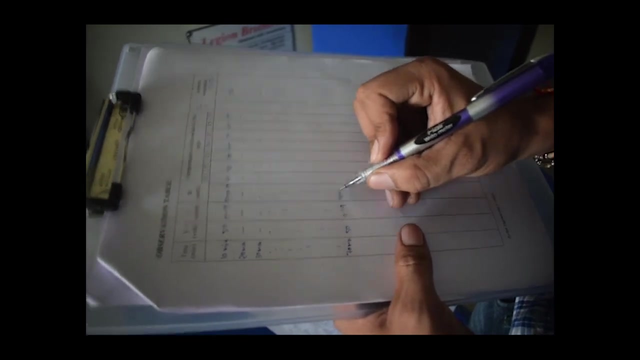 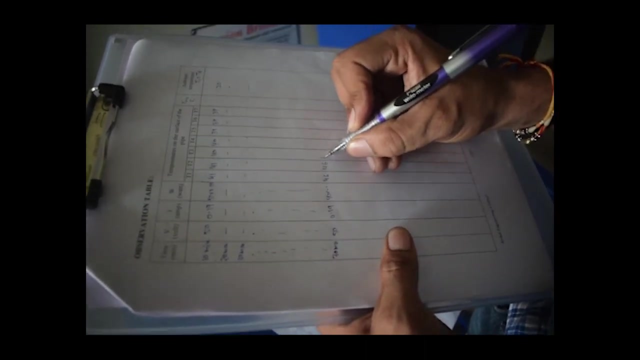 so like that we have to take the reading until the system will not come into the steady state. so supose, after 70 minute, after 70 minute, if i take the reading it will come 50, 50 into 0.9. and i got the reading of first thermocouple. this is suppose 46, this is 46, 45 and 45, 45, 44. 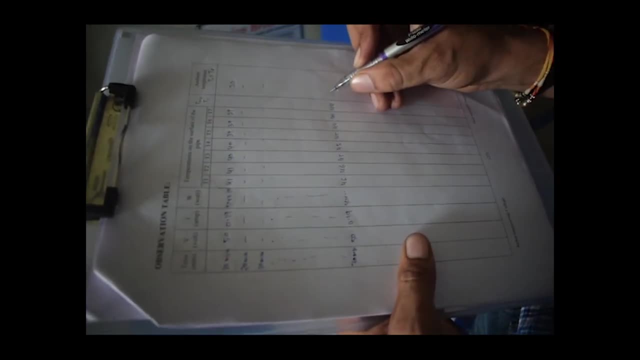 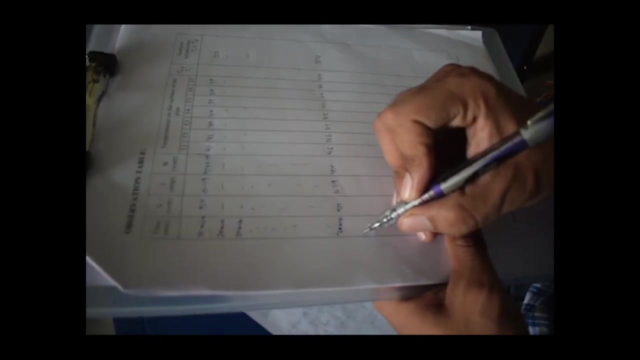 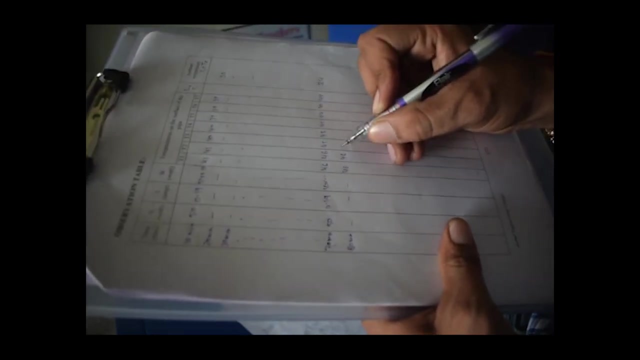 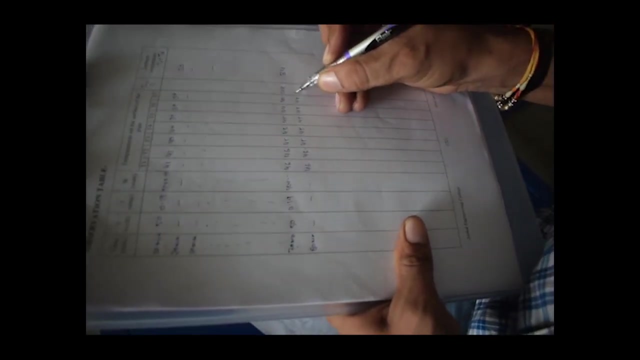 44 and this is also 44 and this is the ambient reading, suppose this is 34. so i got the these, these readings. then again, if i am taking the reading after 10 minute, then i got again these reading 46, 46, like that, 45, 45, 45 and 45 and 34. now we can easily observe that the reading will. 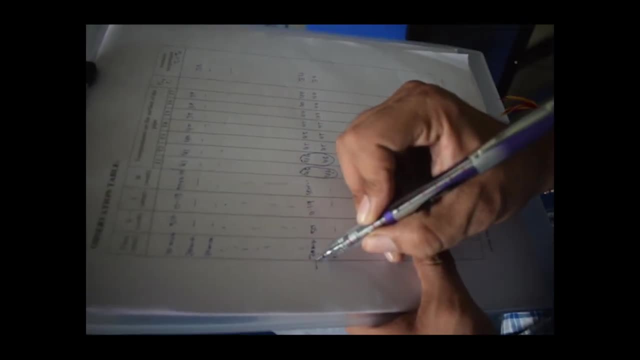 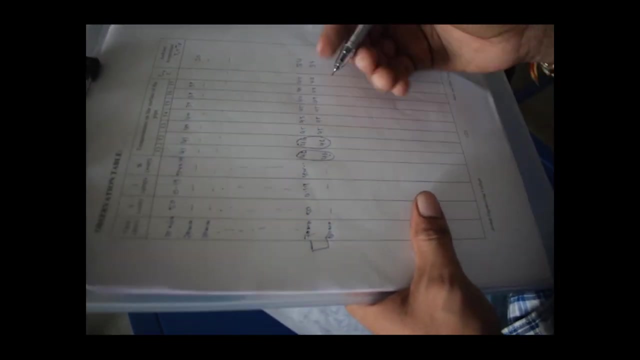 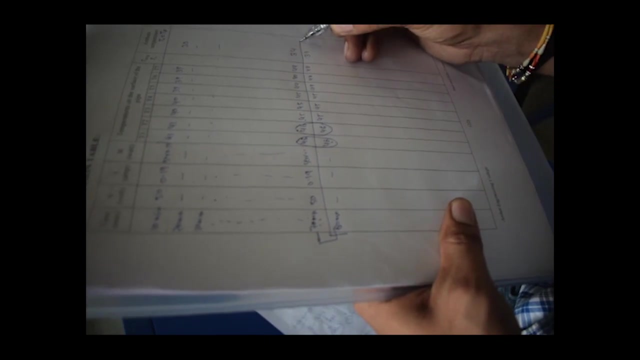 not change. reading will not change with respect to time. that means the system already come in the steady state because the, because the property and the temperature will not change with respect to time. so we will do all the calculation for this reading because these are the readings when the system come in. 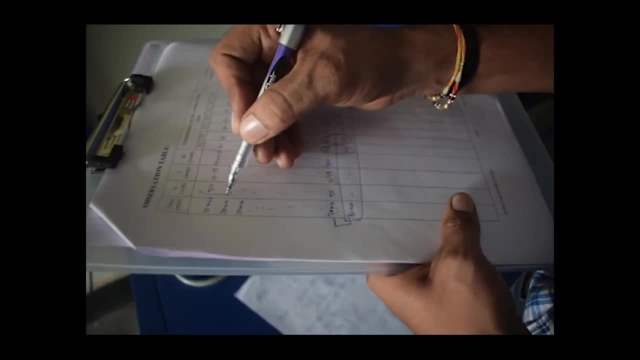 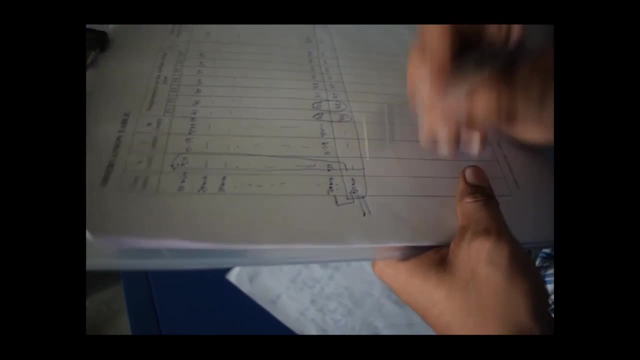 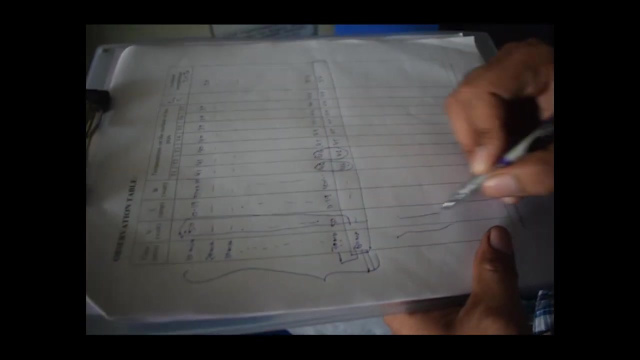 steady state. so all the reading, we take all the reading at same power input, all the reading for the same power input. this is the first observation. if you want to take the reading on another power input, then repeat the same procedure and note down the reading. then again we got the second reading. 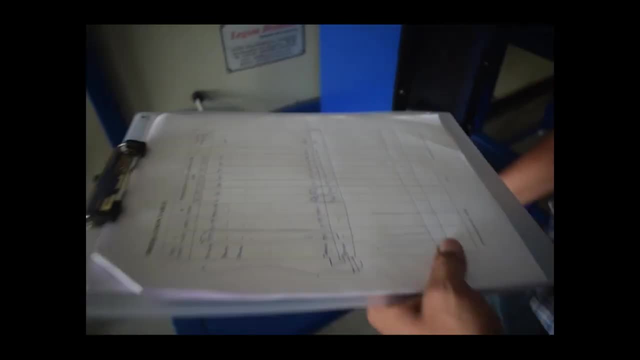 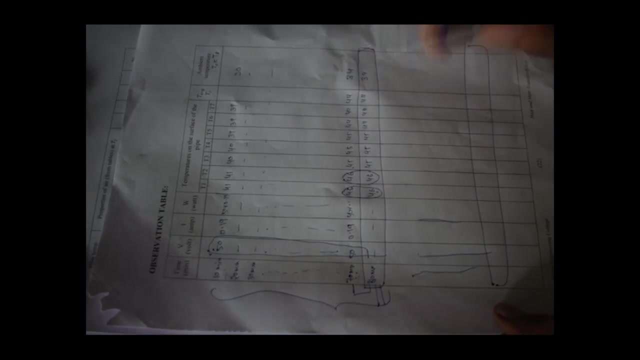 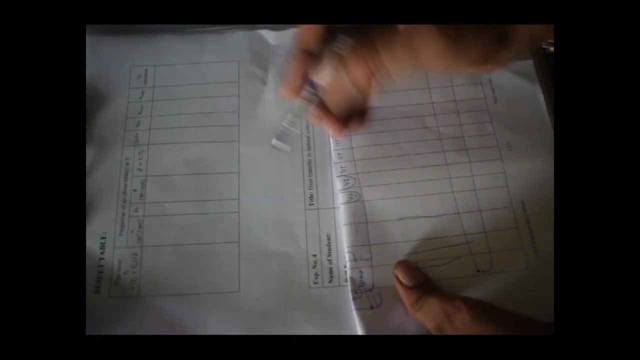 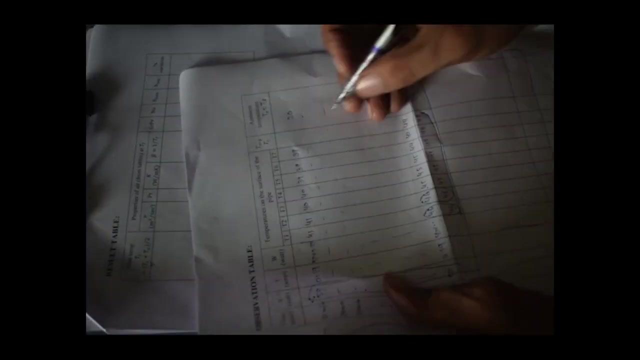 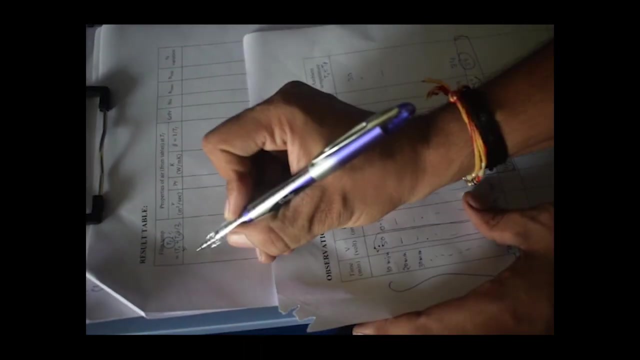 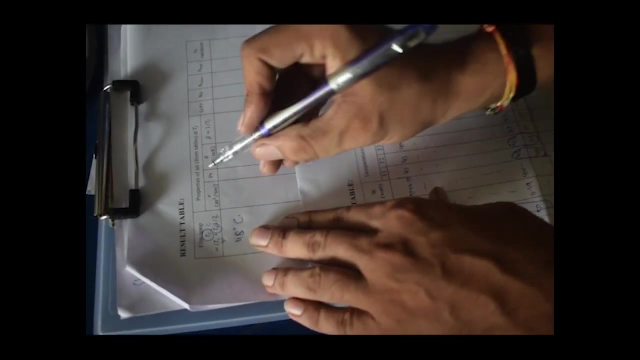 like that, ok. ok, so we get the reading for the steady state condition. so now we can do our calculation. ok, so by averaging this we got the ts, and t8 will give the ambient temperature degree Celsius. So at this temperature from the, from the table properties of table, we get the.